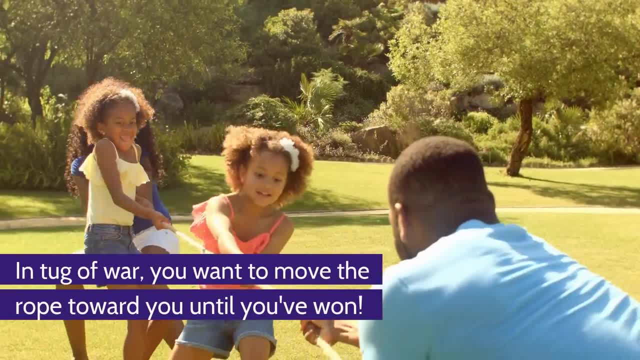 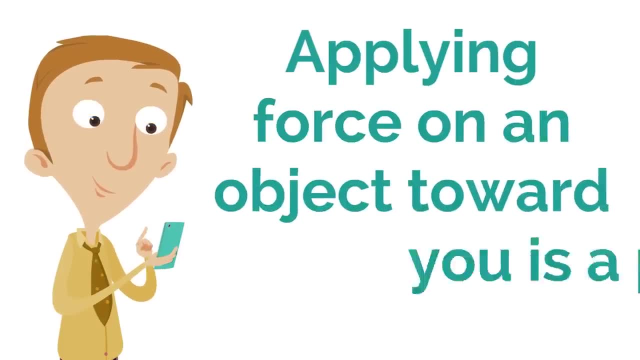 In Tug of War, you want to move the rope toward you until you've won. It's all about moving the rope. Applying force on an object toward you is a pull. Pulls bring objects toward you. That's what a pull is. 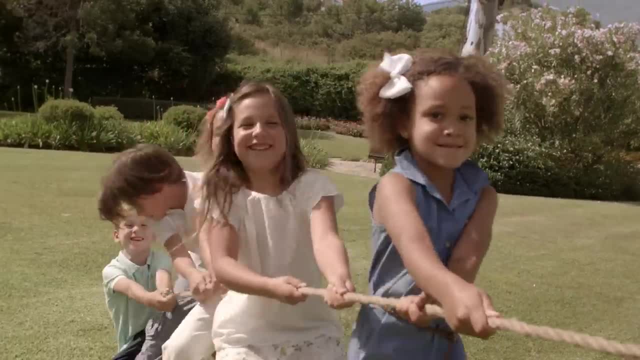 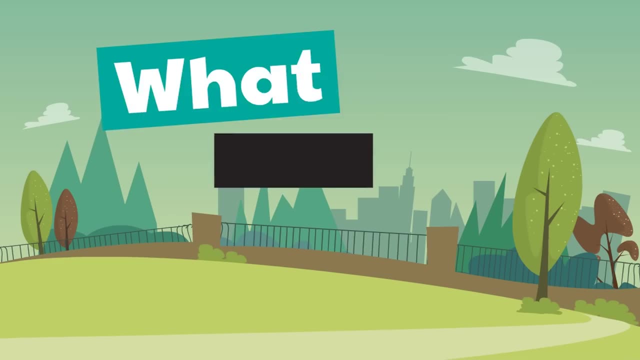 Here the children are pulling on the rope. They are moving the object toward them. They're moving the rope toward them, aren't they? Yes, So what are pushes? Well, a push is the opposite. Pushes move objects away from you. 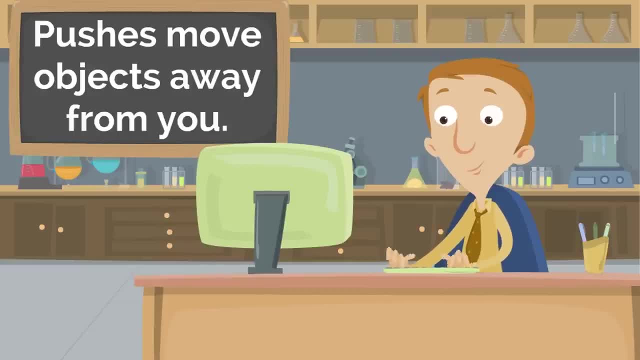 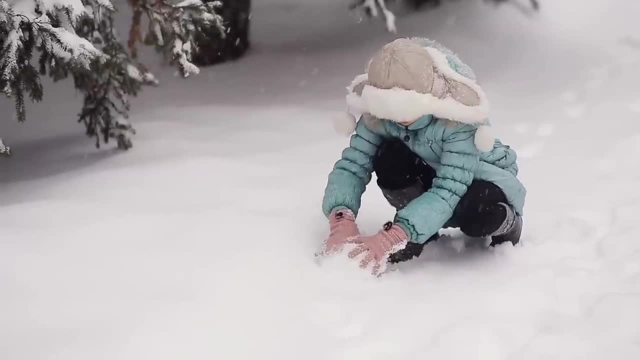 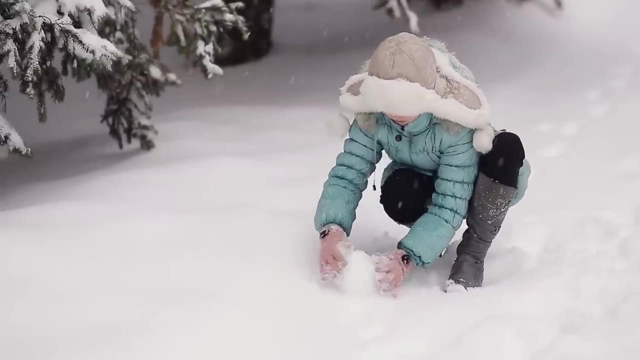 Can you say that with us Pushes, move objects away from you. Fantastic, Wow. do you know what this girl is doing? Uh-huh, She is building a snowman, But she is just just getting started. Whoa, look how big this snowball has gotten. 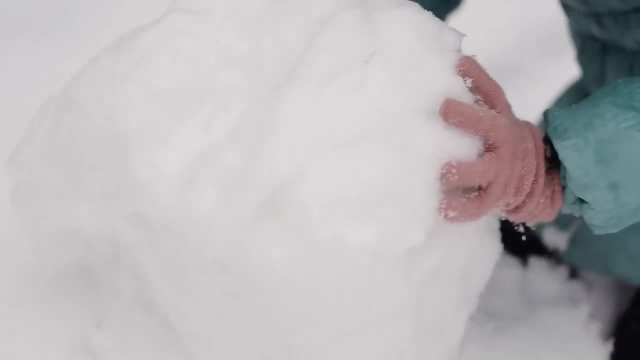 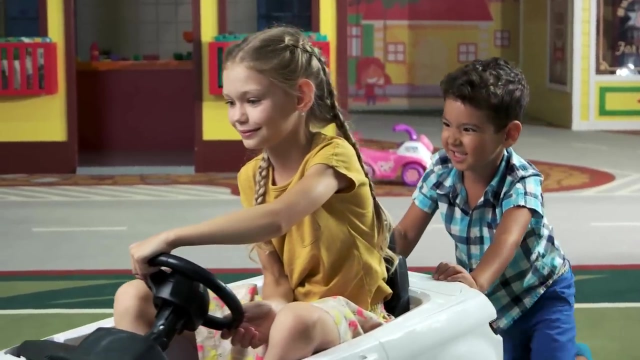 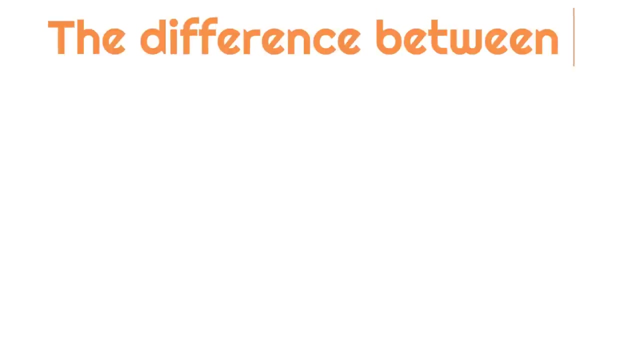 She is using force to move the ball away from her. These are called pushes. She is pushing the snow along. Here is another push. This boy is pushing this girl in a car. Pushing can be hard work. The difference between a push and a pull is in the direction it is going. 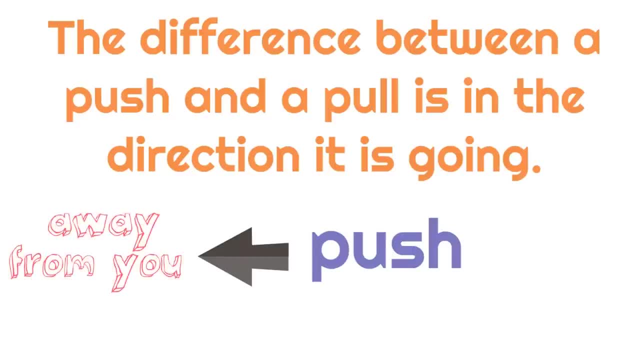 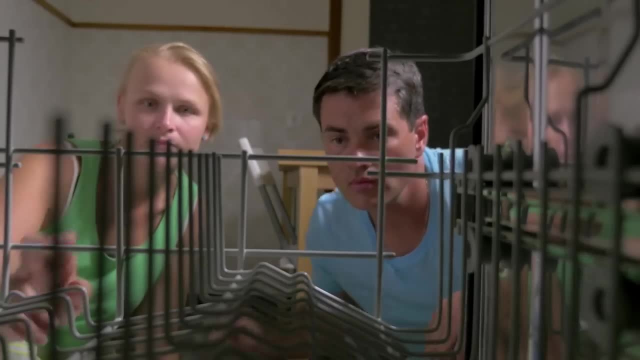 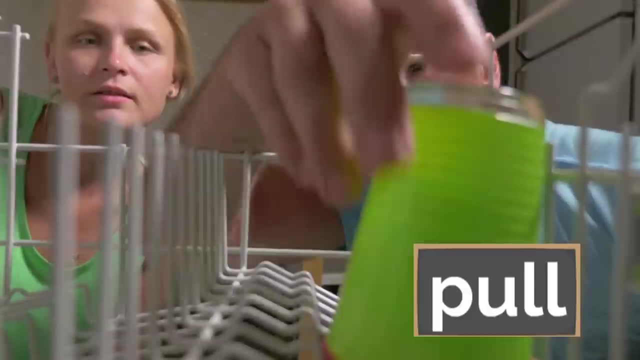 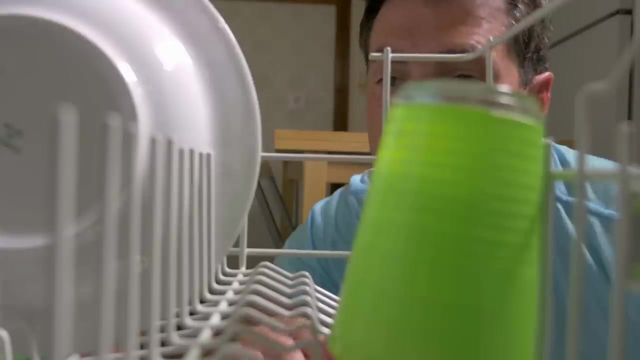 A push moves an object away from you. A pull moves an object toward you. You try now. Is this a push or a pull? Yes, a pull, Because they applied force to move the rack toward them. This is a pull. Okay, so we're just gonna watch them load up dishes, huh. 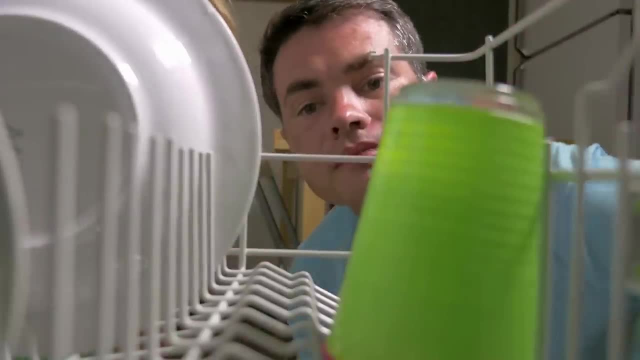 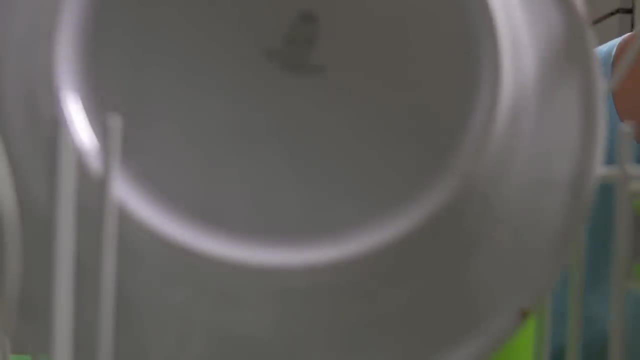 Okay, this is getting gross. Okay, uh-oh, Is there more? Oh this, Oh, we can't even see. Oh, there's a crumb there, We can't even see. Oh, don't close the door. 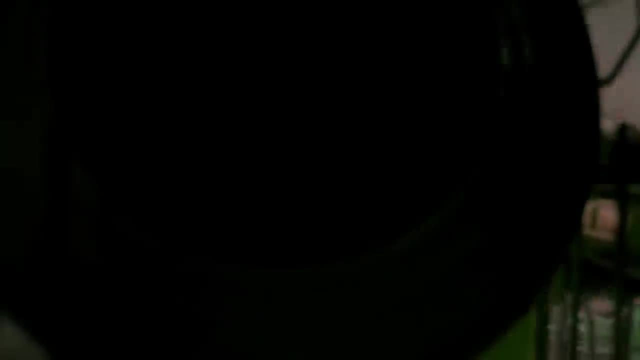 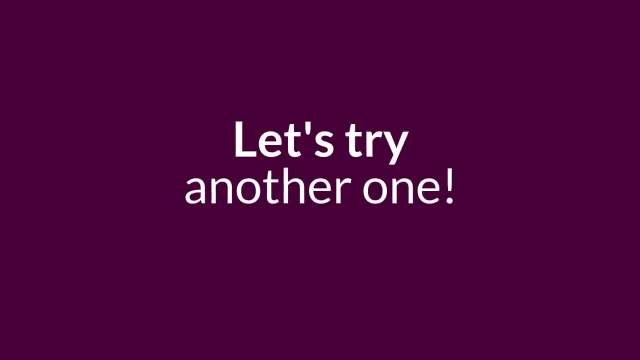 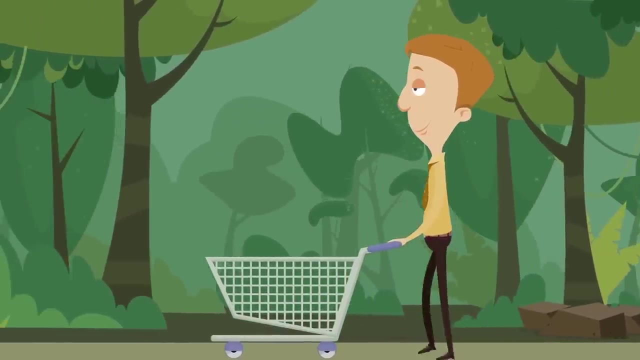 Don't shut us inside the dishwasher, Don't. Alright, let's try another one. That got a little intense. Am I pushing or pulling? Is this a push or a pull? Notice, I have to keep walking to keep up with it.